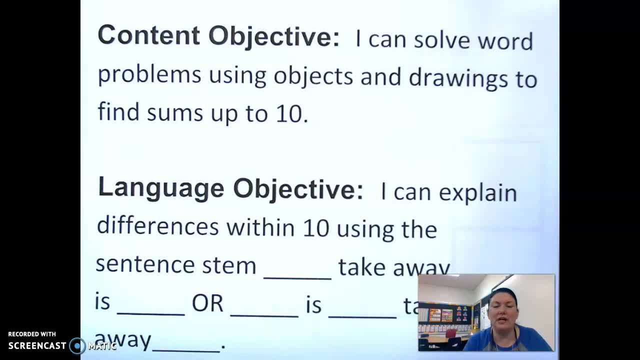 And so if you need a little bit of time to gather your materials, please pause the video and do that now. Otherwise we're going to go ahead and move on to today's content and learning objective. Today's content objective says: I can solve word problems using objects and drawings to find sums. 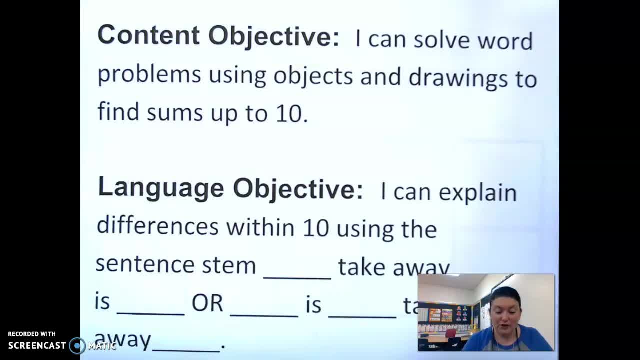 up to 10.. Well, first of all, Ms Lankford has made a mistake, And you know what? That is okay, because one of the habits of a math teacher is to make sure that they're not making mistakes- Is that mathematicians make mistakes? Today, we are working on subtraction, So we are not working. 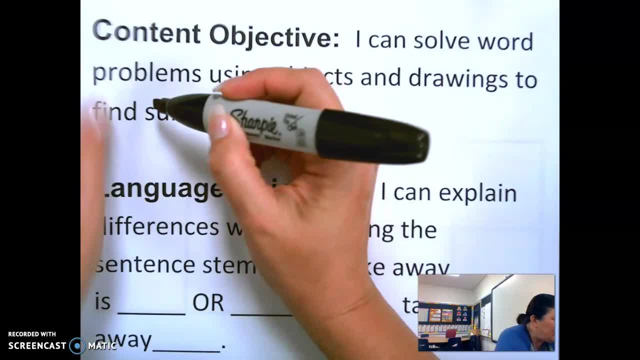 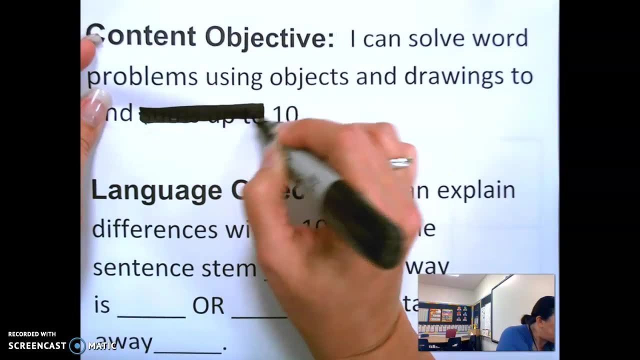 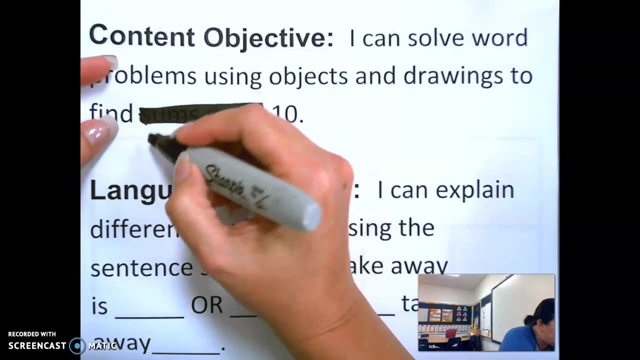 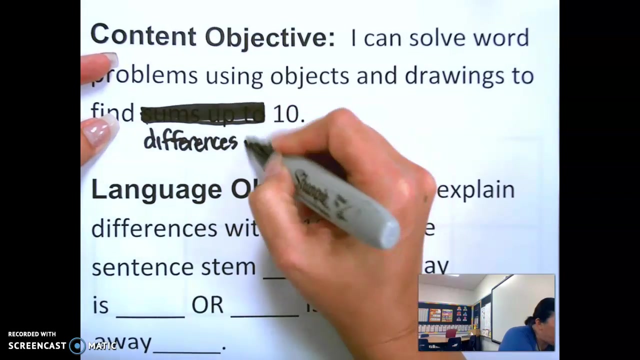 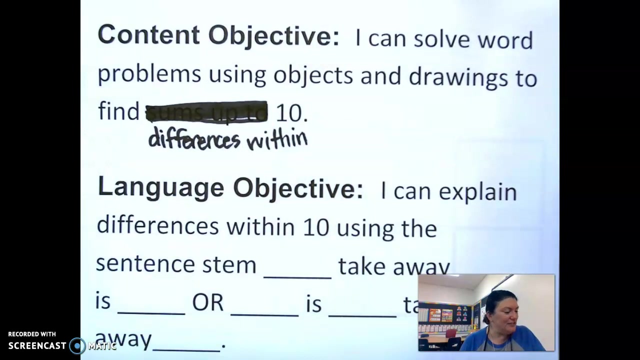 on sums, boys and girls. We are working on differences Differences. So I'm just going to take this, I'm going to cross that out And I am going to replace that with differences Differences- Differences Within 10.. Oh, it's kind of hard to write this way, but that's okay. Differences within 10.. And 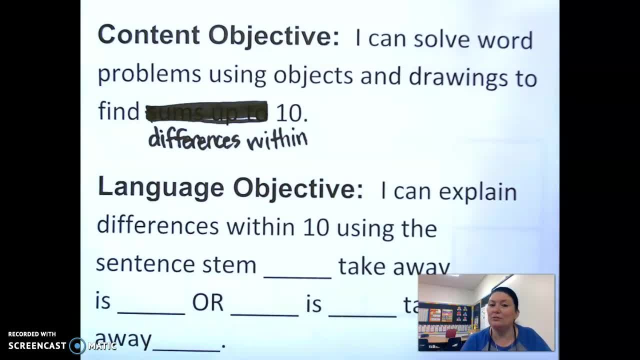 remember, differences are the answers to a subtraction problem. Again, mistakes are just one of the habits of a mathematician. We learn from them and it makes us stronger at math. So again, our language objective now states that I can explain differences within. 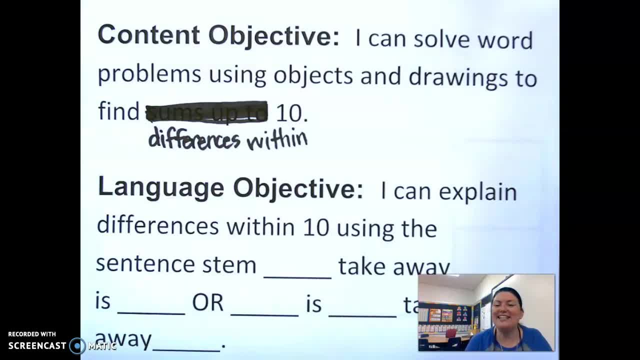 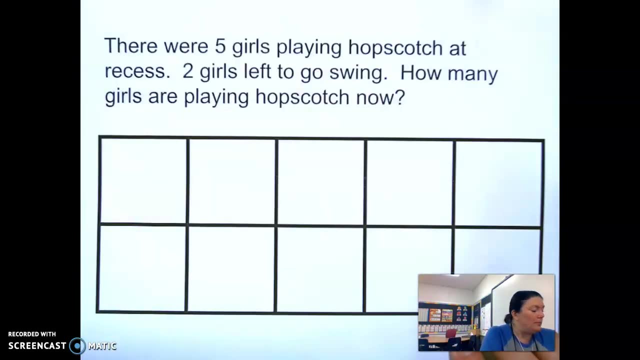 in 10.. I got it right that time, Using this sentence: stem blank, take away blank is blank, or blank is blank, take away blank. So let's get started. Remember that a word problem is simply another name for a math story. So our first word problem says that there were five girls playing. 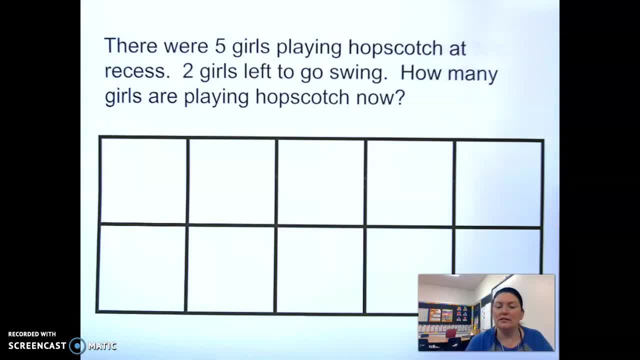 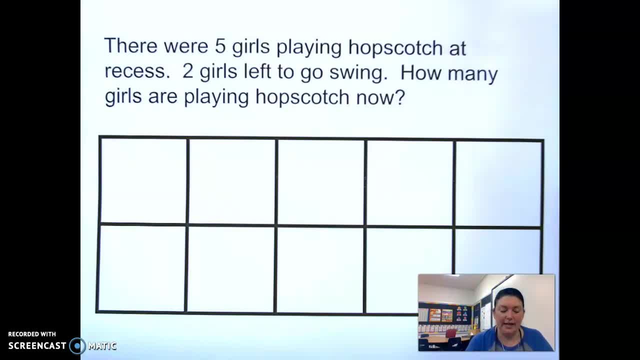 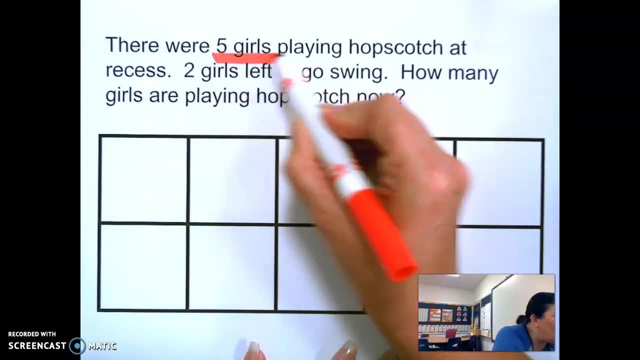 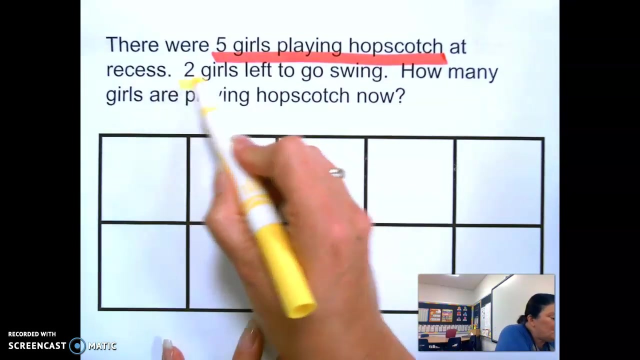 How many girls are playing hopscotch now? Well, just like I did with my addition stories, I'm going into my problem first and I'm looking for the things that I already know. I already know that five girls were playing hopscotch. I also know that two girls left to go swing My story. 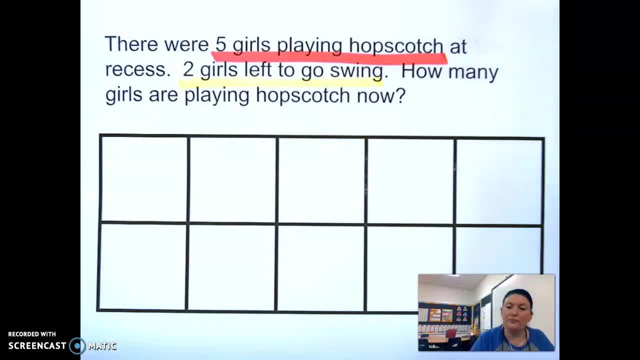 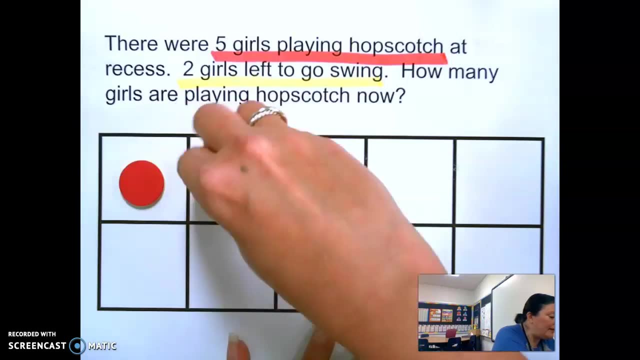 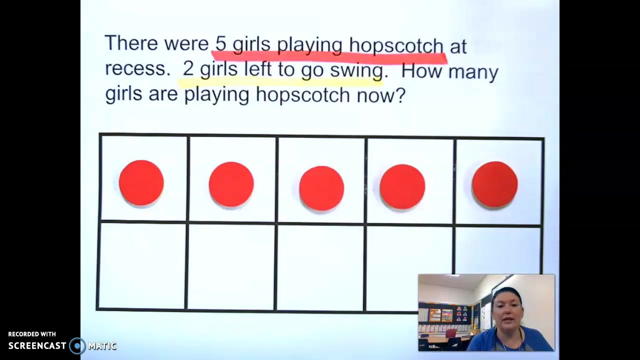 asks me how many girls are playing hopscotch now. So in order to solve my problem- my word problem of differences within 10, I'm going to represent that problem with counters. So I'm going to start with my five girls playing hopscotch Now. you'll notice that Ms Langford did not go through and 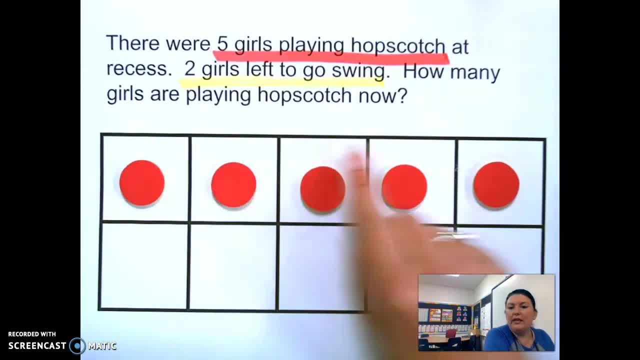 say one, two, three, four, five, six, seven, eight, nine, ten, eleven, twelve, twelve, thirteen. I didn't have to do that because, if you remember, just like we talked about in our addition lesson. 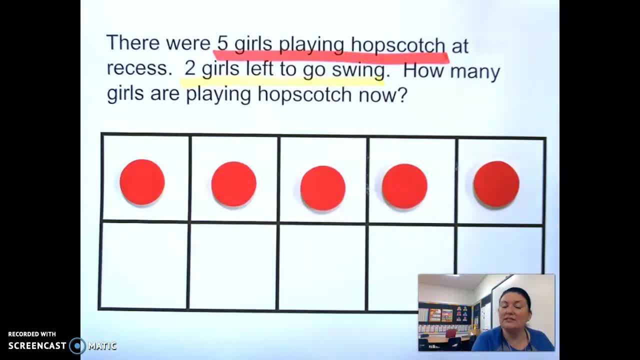 the top row of our tens frame has five places, So I already knew that I just needed to fill up that row if I wanted to represent my five girls playing hopscotch. Now my story also tells me that two girls left to go swing. Now it doesn't matter which two girls we pick, but Ms Langford's going. 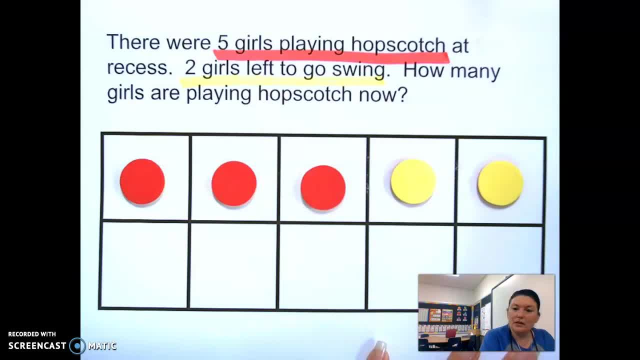 to pick the two girls that are left to go swing. Now Ms Langford's going to pick the two girls that are right here at the end. those two girls left to go play on the swings. they were tired of playing hopscotch. their legs wanted some rest. they wanted to go swing and feel the air. 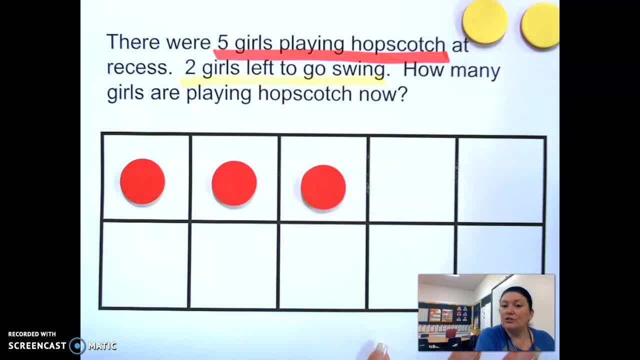 and enjoy the swings for a little bit. so how many girls were left playing hopscotch? three, you're right, we have one, two, three girls left playing hopscotch. so i'm going to show you now what that's going to look like if we were going to model that using a drawing, or try to. 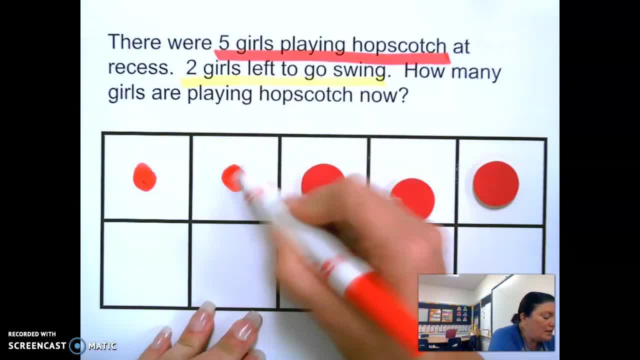 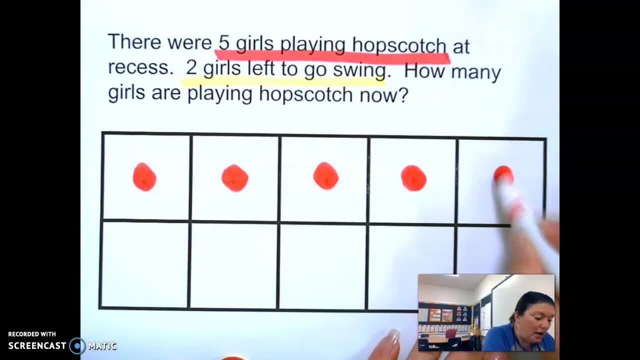 solve that using a drawing. remember, when i'm using a drawing as my representation to solve, i'm simply replacing my objects with a picture. so there's my drawing. so there's my drawing. my five counters and two of my girls went to go swing. Now Miss Langford's going to choose to use. 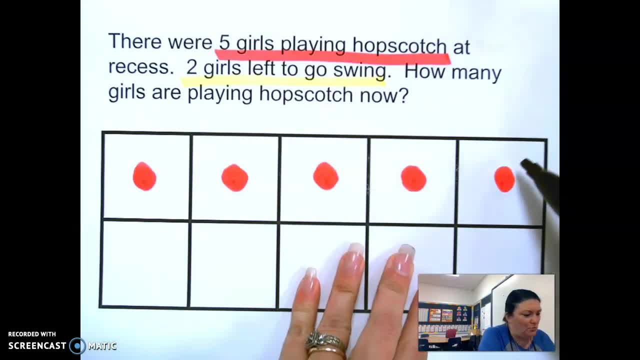 her black instead of her yellow, because I don't want to mess up my yellow marker. Sometimes, you know, when we use yellow markers they get other colors on them and I don't want to mess that one up, So I'm going to use black. So those two girls left to go swing. So if I cannot count these, 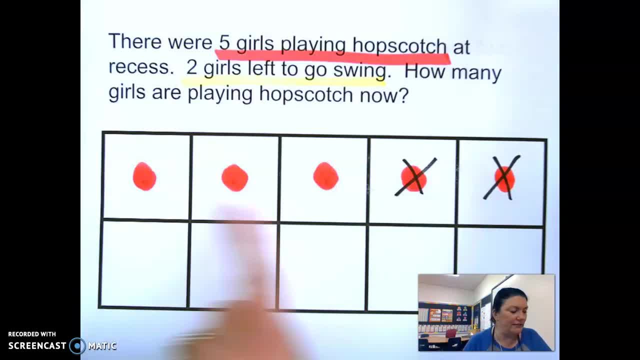 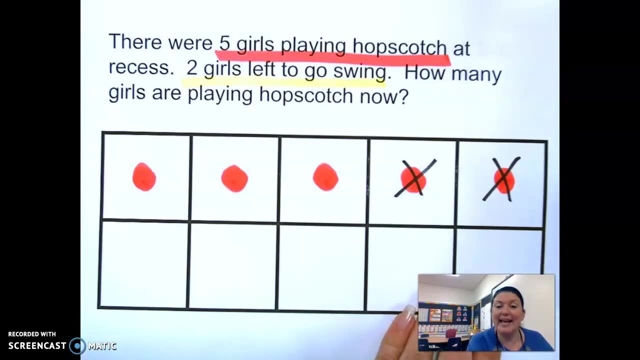 because they have X's on them. how many girls do I have left playing hopscotch? You're right, I still have three. So it doesn't matter if I'm using my objects or a drawing. I can still solve my problem and use my sentence stems to say five. take away, two is three. I could also say three is five. 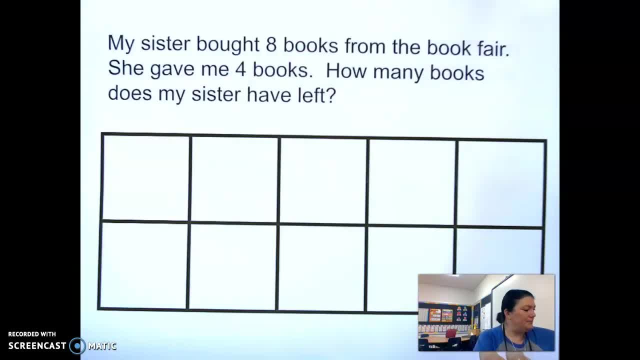 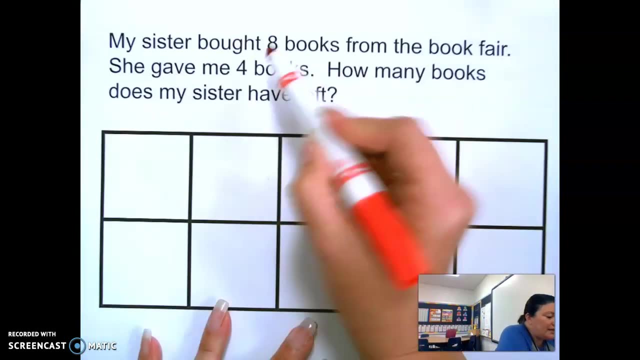 take away two. Let's look at another example. Let's look at another one. My sister bought eight books from the book fair. She gave me four books. How many books does my sister have left? So I know that I, that my sister bought eight books from the 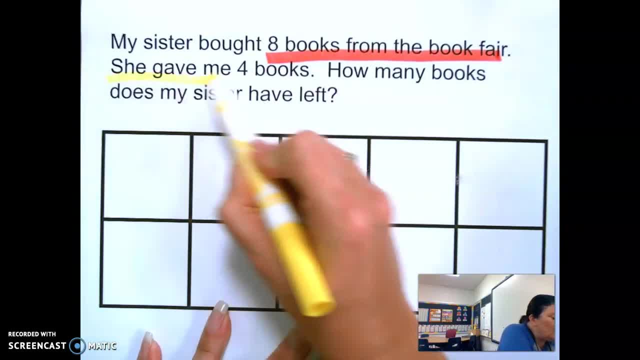 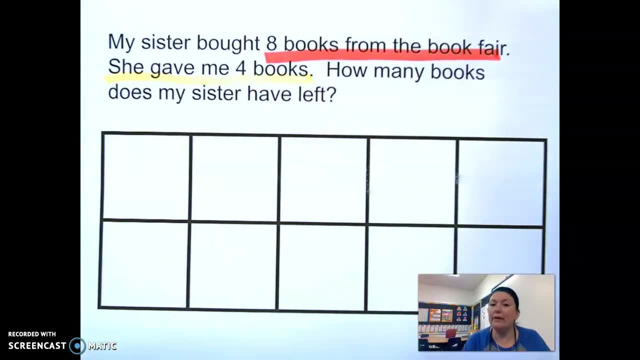 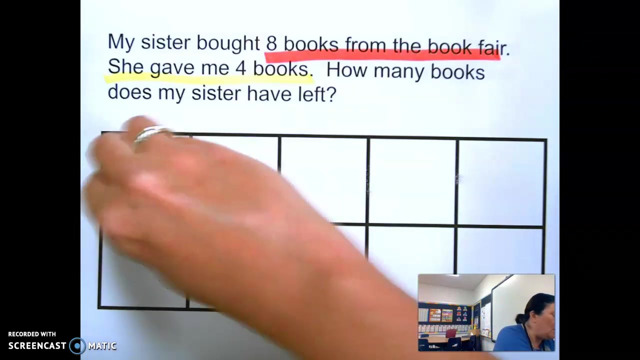 book fair. I also know that she gave me four books, So she separated her books. She separated those books into- And here is another example: Ten or twelve books from the book fair. Hello everybody, I just want to take a second and just think of the answer. She bought eight books from the book fair. So let's try. 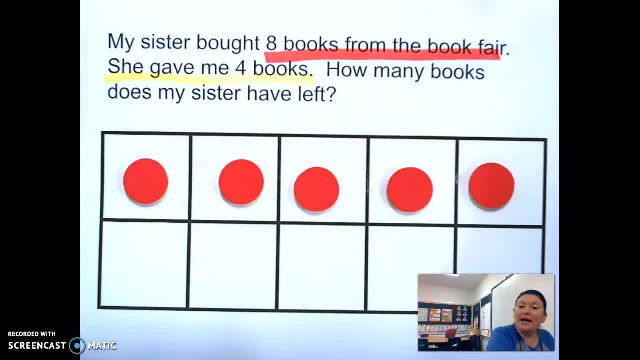 put a number into the book fair, So I think times seven now, if you see, by manyử estate and not so many то всё lol. was it nice? Yes, it's always nice to share. So let's see how we can model that using our objects. I'm going to be using counters, you might. have counters. you may have something else. So let's start with eight books. We know that she bought Tiga, http//lnbworldcom. eight books- and again I'm not counting these by ones, because I know this is five- and these books. 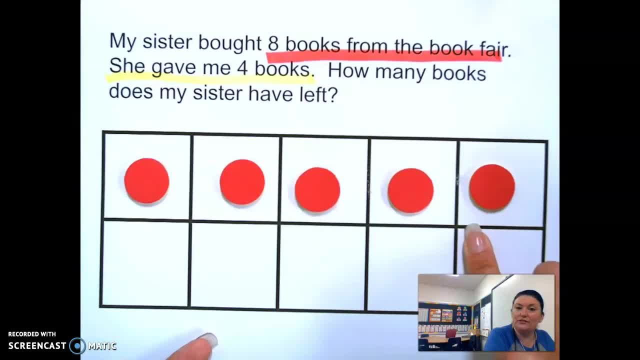 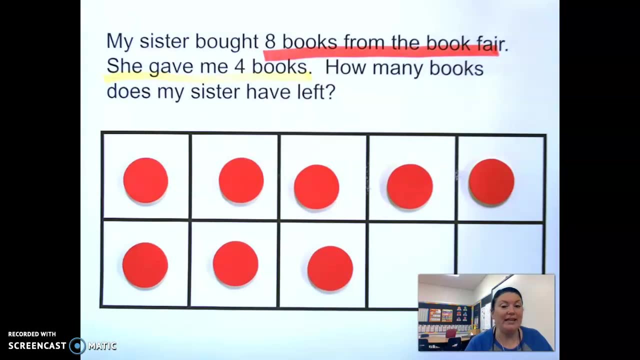 are underground. These are, notiration, Brazilian books only. but five books are 그� c hate per case. this is an know. this is five if i filled up the top row, so now i can just count on from five, six, seven, eight. that is an efficient way that a mathematician works. we can count on from five, so now that i 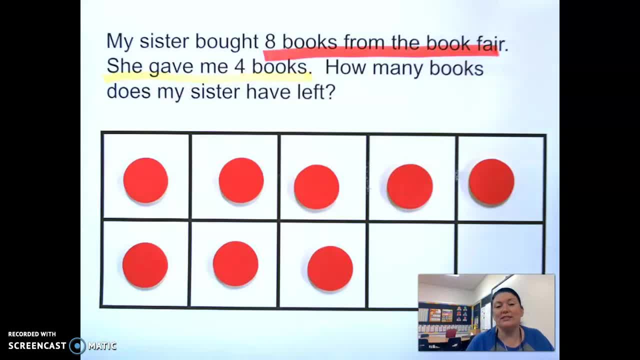 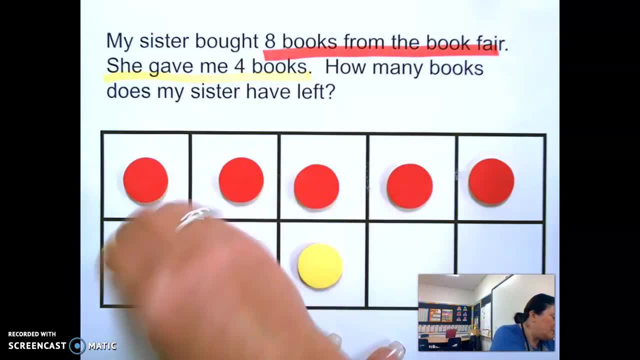 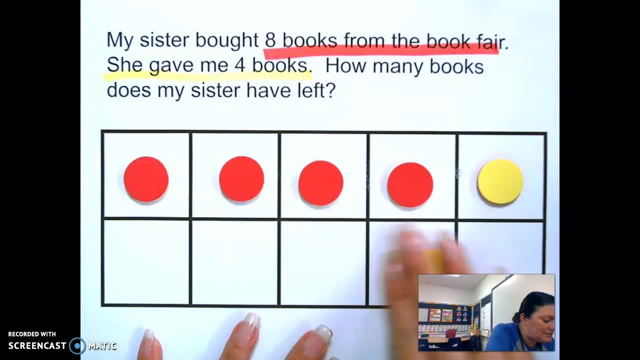 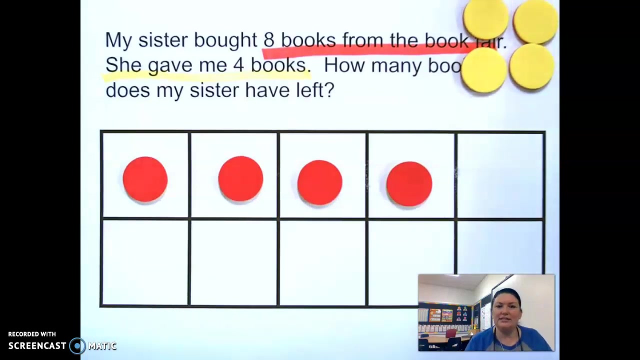 have my eight books there. my sister was kind enough to share with me and she gave me four books: one, two, three, four. so if she took these four books and she gave them to me, how many books does my sister have left? four, she also has four. one, two, three, four. so we could use our sentence. 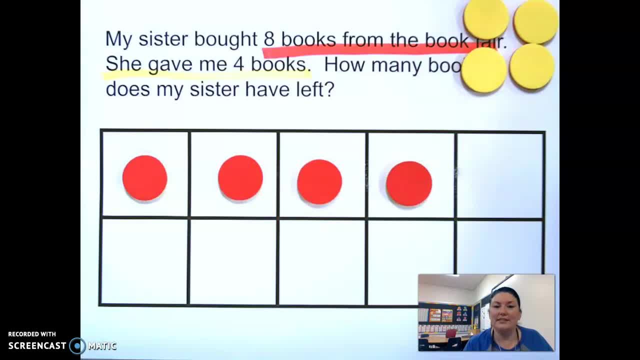 stem and say four, take away. i'm sorry there goes, miss langford, with that mathematician mistake. again. i'm looking at the numbers on the screen and i'm reading ahead of myself. i could use my sentence stem to say eight, take away. four is four. i could also say that four is eight, take away four. 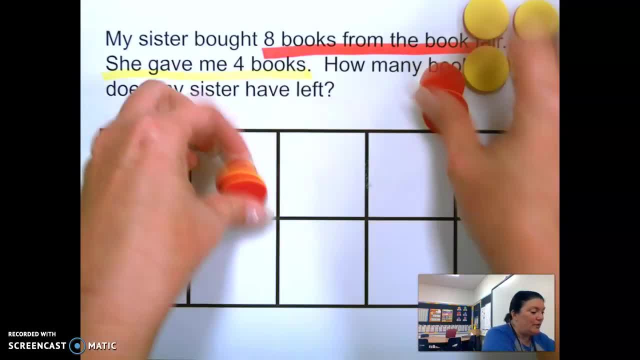 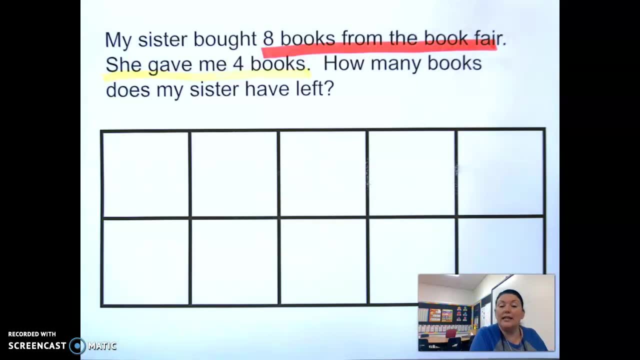 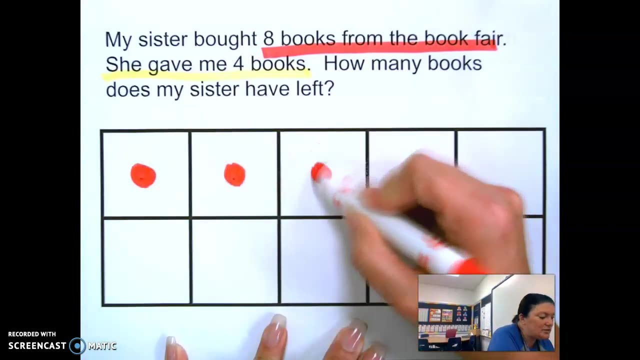 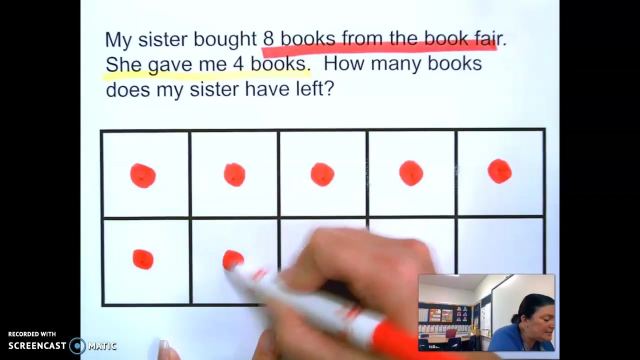 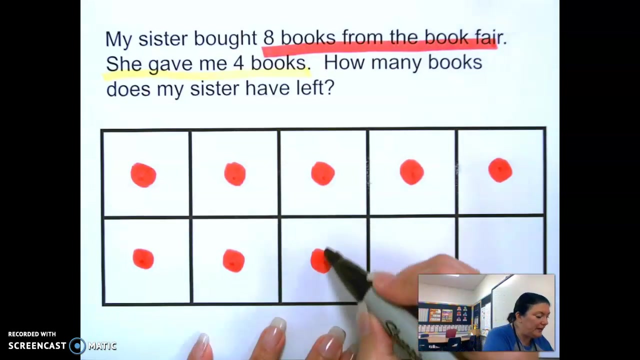 either way is correct, boys and girls. so if i'm using this same problem to uh use, to model it in a pictorial representation or in a drawing, i would still start with my eight books, by putting in five in the top row and then counting on six, seven, eight. there's my eight books that my sister bought from the book fair. 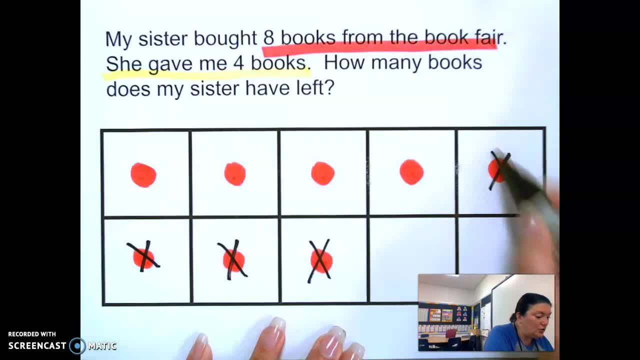 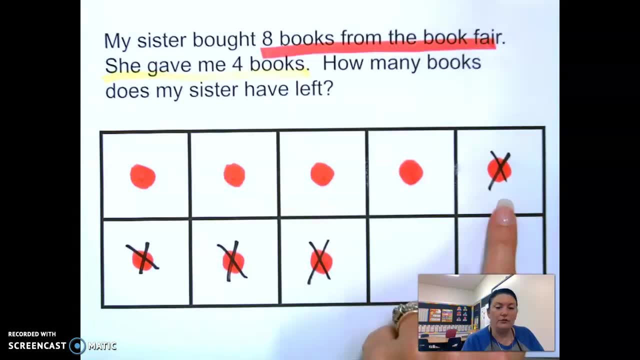 she gave me four, so i'm going to cross off the four books that she gave me: one, two, three, four. is this not the same thing that we just did with our counters? absolutely so. even if you don't have counters, as long as you have something to write with, you can still solve your problem. 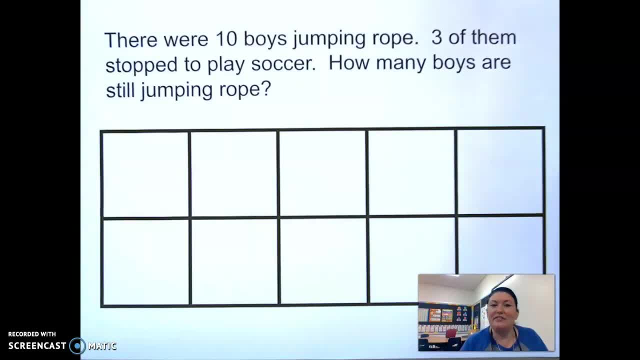 and our last problem for today says that there were 10 boys jumping rope. three of them stopped to play soccer. how many boys are still jumping rope? so again, the first thing i do is i go into my problem, i look for what i know, and i know that there were 10 boys jumping rope. i also know that three of them stopped to play soccer. 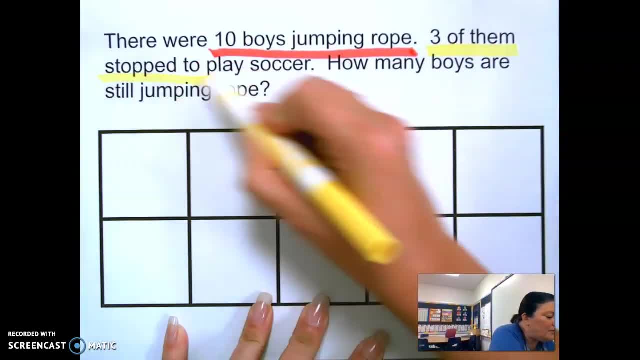 i also know that three of them stopped to play soccer. so, again, the first thing i do is i go into my problem. i look for what i know, and i know that there were 10 boys jumping rope. i also know that three of them stopped to play soccer. 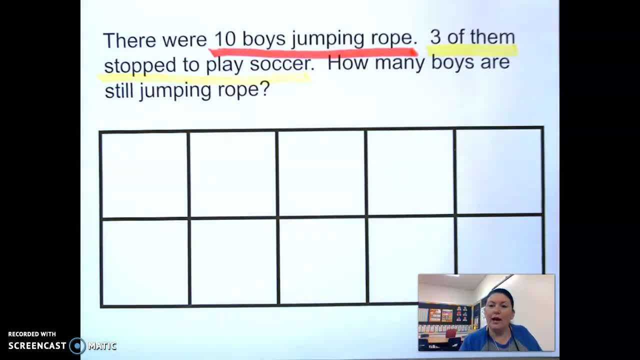 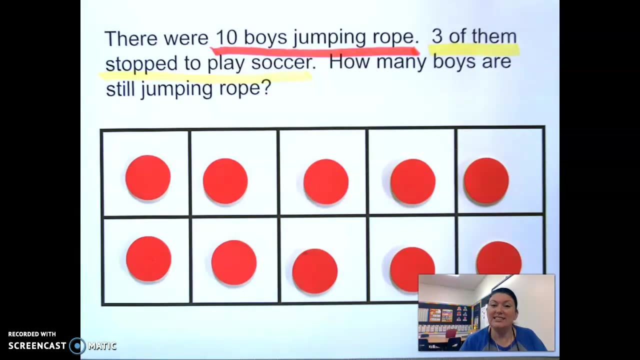 stopped to play soccer, So I'm going to use my counters to represent that And I want you to watch, because Ms Langford is just talking. I'm not really even counting at all. All I'm doing is putting those counters in the tens frame. Does anybody know why I didn't count those? 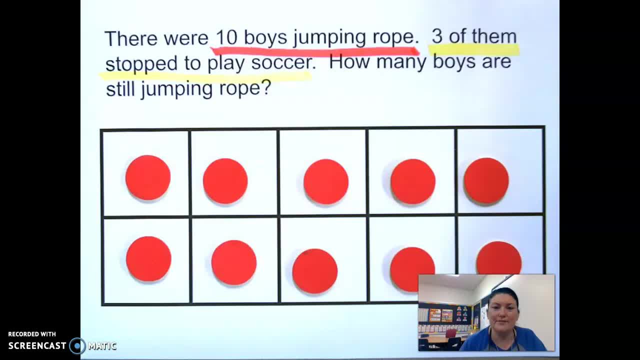 You're right, A ten frame already has ten spots. So if there were ten boys, I know that all I needed to do was put one counter in each of those spots. I didn't have to count one, two, three, four, five, six, seven, eight, nine, ten to know that that was ten, because a ten frame 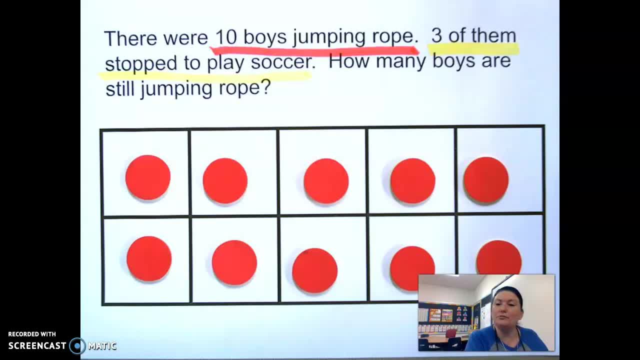 already has ten spots. So if there were ten boys, I know that all I needed to do was put has ten spaces. I filled my ten frame up with ten counters, So I've represented my ten boys that are jumping rope. But remember my story also tells me three of them stopped playing soccer. 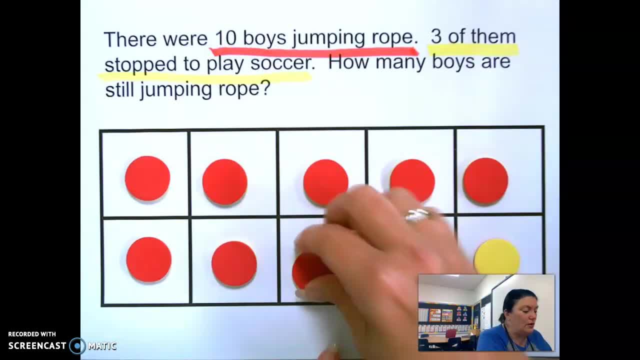 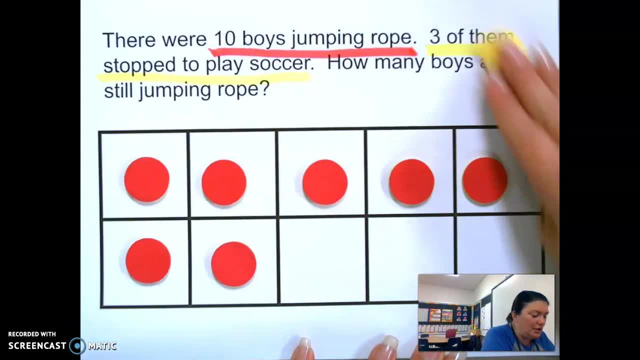 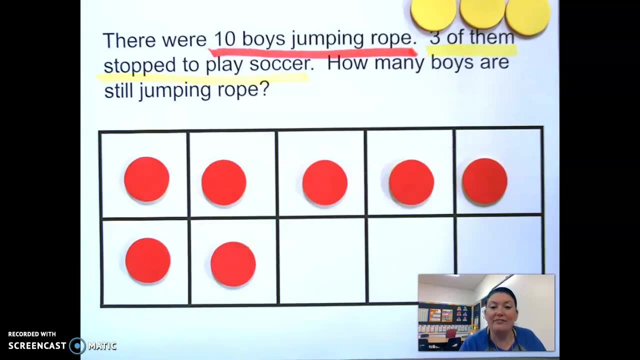 I counted one, two and three. These three boys ran off. They were like: nope, we're done playing jump rope, We want to go over here and play soccer. I'm going to go over here and play soccer. We're going to move them out of the way. And so now I have how many boys left? 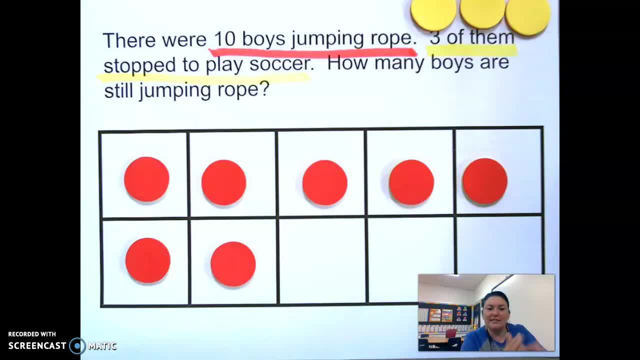 Seven. If you said seven, you are correct. Give yourself a round of applause. We know that this is seven because we already know this is five. We counted on six, seven, or maybe we counted them one at a time: One, two, three, four. 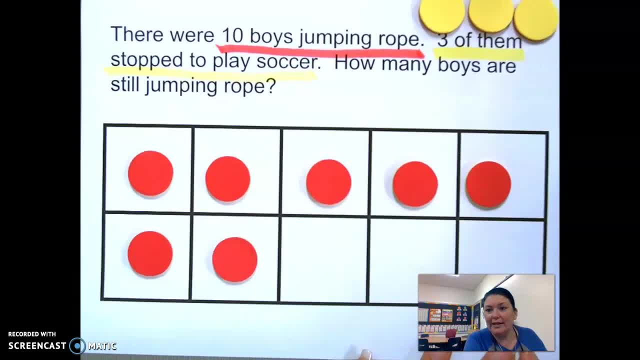 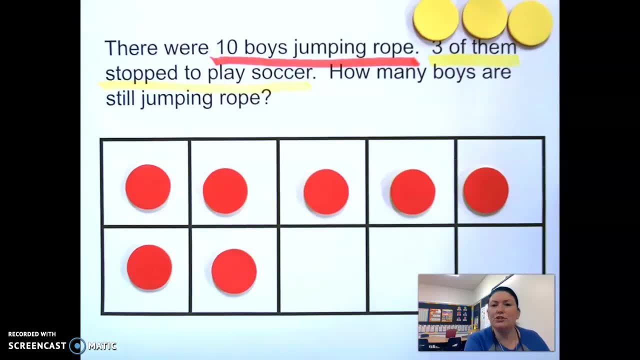 six, seven. either way is correct. miss Langford just likes to show you the more efficient way of doing that, and so using my sentence stems. why don't you try to say it with me? let's use the first sentence: stem. ten, take away. three is seven. can you say that with me? ten, take away. 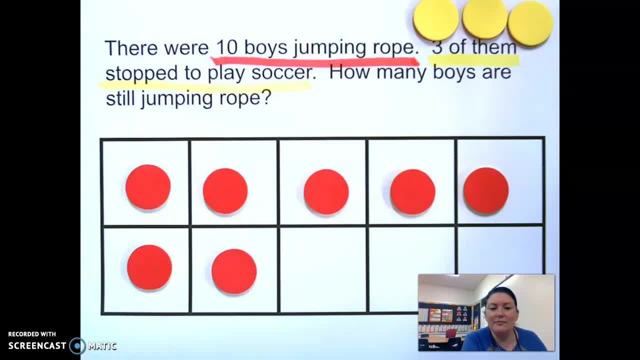 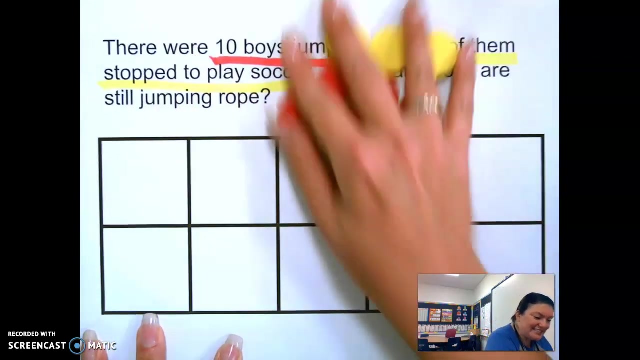 three is seven. now let's try it with our second sentence: stem, seven is ten, take away three. say it with me: seven is ten, take away three. either way is correct. lastly, we are going to use a drawing to solve this problem. we're going to do it the exact same way. we're going to do it- the exact.